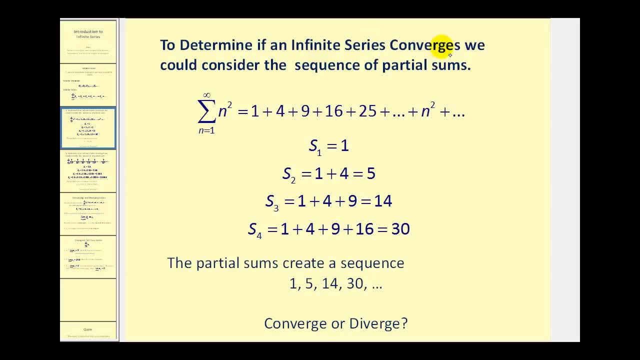 So to determine if an infinite series converges or diverges, we must consider the sequence of the partial sum. So what that means is, if we have an infinite series here, if we want to know if it converges, we're going to take a look at the sum of the first term, which would be just 1,. 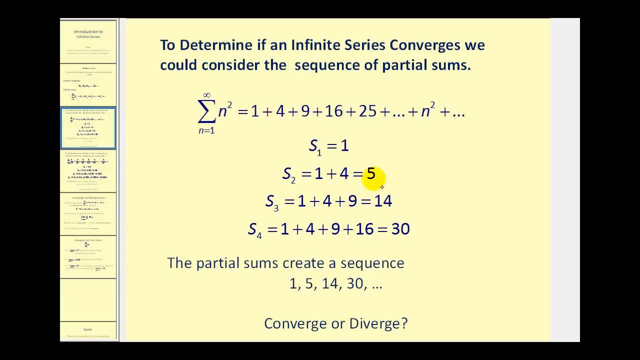 the sum of the first two terms, which would be 1 plus 4, which equals 5, the sum of the first three terms, which would equal 14, and so on. And the question becomes: does the sequence of the partial sums 1,, 5,, 14, and 30 converge or diverge? 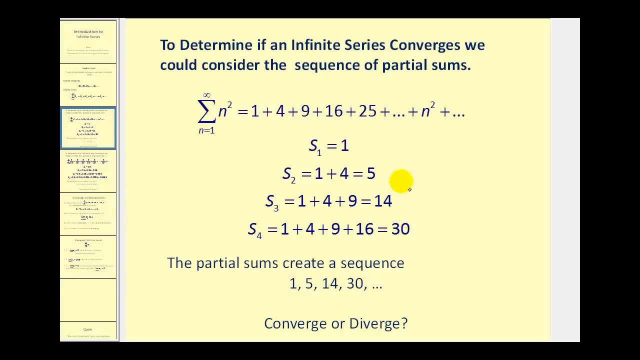 So the sequence of the partial sums 1,, 5,, 14, and 30 converge or diverge. This sequence is generated by the partial sums of the infinite series And it's probably pretty easy to see from this sequence. it appears as if this is going to increase without bound and therefore this infinite series diverges. 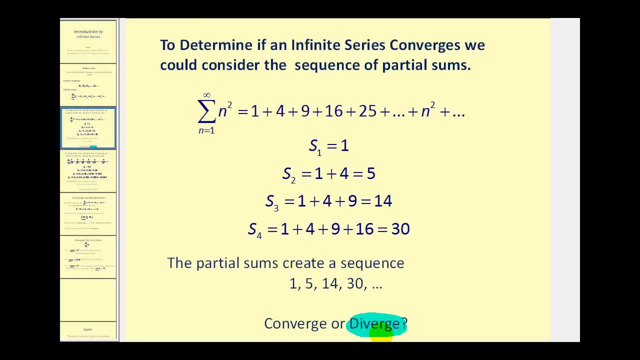 We'll take a look at a more formal definition in a few minutes. Let's go and take a look at another infinite series. Here we have the infinite series of 3 divided by 10 to the power of n. So when n is 1, we'd have 3 divided by 10 to the first. 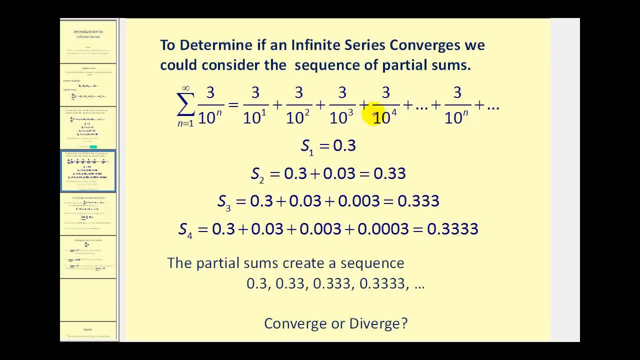 When n is 2,, we'd have 3 divided by 10 to the second, and so on, And then we'd find the sum of these terms. Let's take a look at the partial sums in decimal notation. Well, the sum of the first term would just be 3 divided by 10, or 3 tenths. 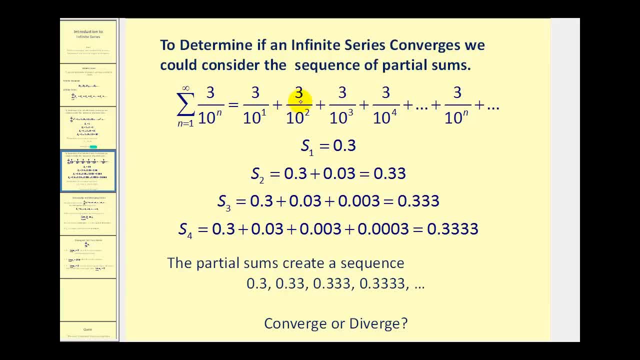 The sum of the first two terms would be 3 tenths plus 3 hundredths, which would be .33.. And then the sum of the first three terms would be 3 tenths plus 3 hundredths plus 3 thousandths, as we see here in decimal form, which is 0.333.. 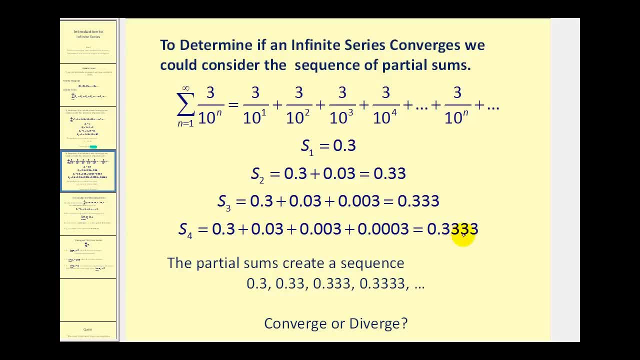 And you can see, the sum of the first four terms would be 0.3333.. So the question becomes: does the sequence created by the partial sums, as we see here, converge? It looks like this 3 is going to repeat forever. 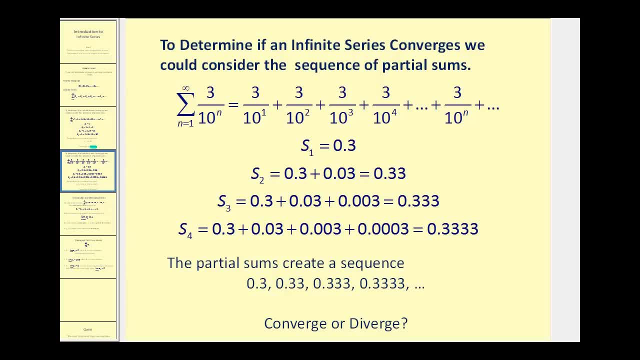 And 0.3. repeating should remind you of the fraction 1 third. So it does appear that this infinite sum will equal 1 third And therefore we say the series does converge. Let's take a look at a few more examples, graphically as well, by taking a look at this animation. 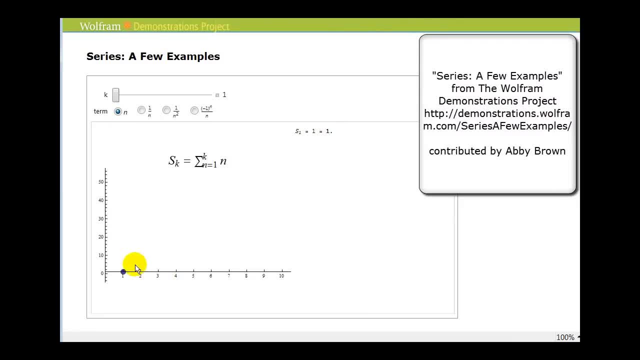 We're going to see the partial sums on the right and then we'll see the graph of the partial sums on the left. So as n increases from 1 to 10, we're seeing the graph on the left and the actual partial sums on the right. 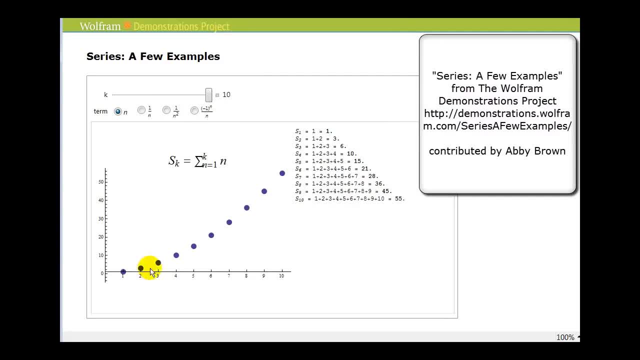 And it does seem pretty obvious from this graph that it is increasing without bound and therefore we would say this series diverges. Now this next series generated by 1 over n is called the harmonic series. It's a very interesting series and we'll take a closer look at this in a later video. 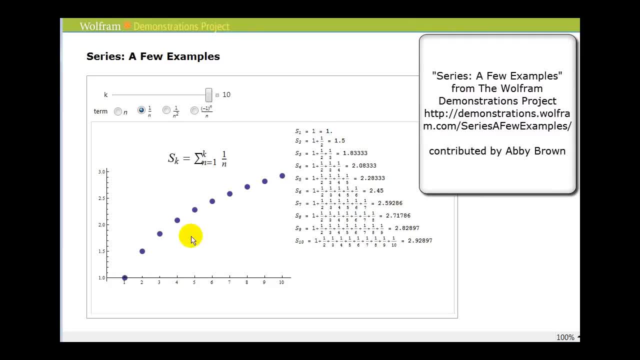 But for right now we're just taking a look at the partial sums on the right and the graph on the left, And it may seem unclear as to whether this series converges or diverges, And we'll come back to this idea in another video. We don't want to spoil all the fun here. 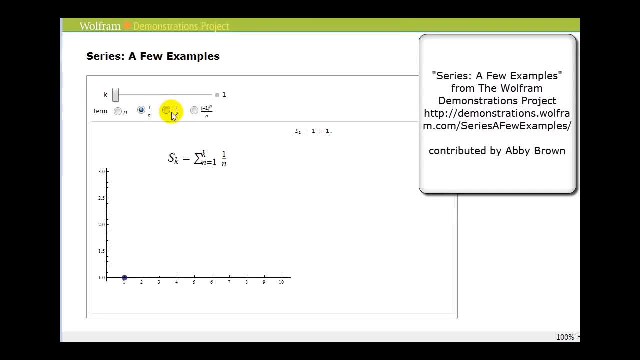 The next series we'll take a look at will be 1 over n squared And again we'll be taking a look at specific tests to determine whether a series converges or diverges in the next several videos And again looking at these partial sums. 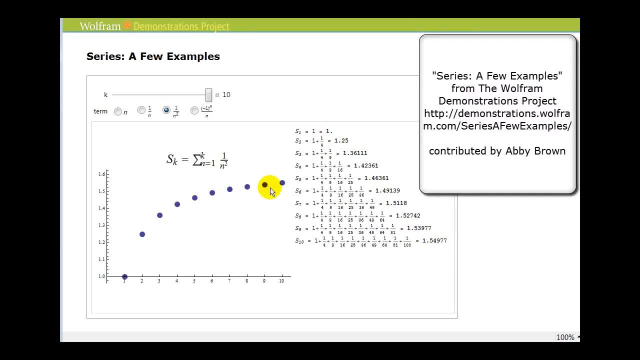 it does appear this series will converge, But again we'll come back to that idea in another video. Let's go and take a look at one more, where the terms in the series alternate sign. And again we're looking at the graph on the left and the partial sums on the right. 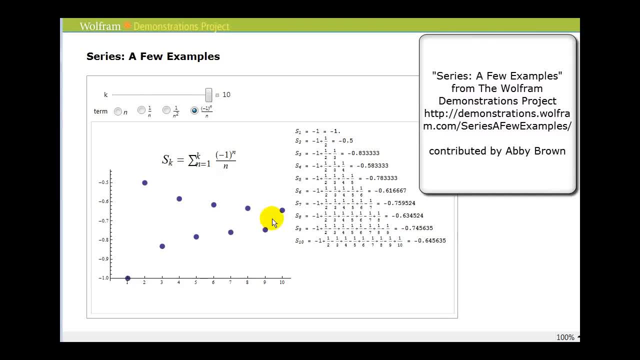 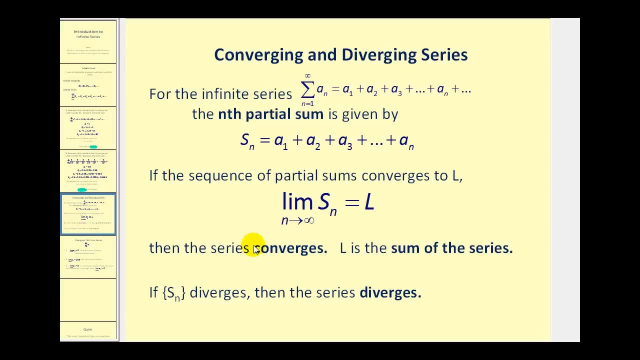 So do you think this converges or diverges? Well, we'll have to wait and see. Let's go and take a look at a more formal definition of converging and diverging series For an infinite series, as we see here. 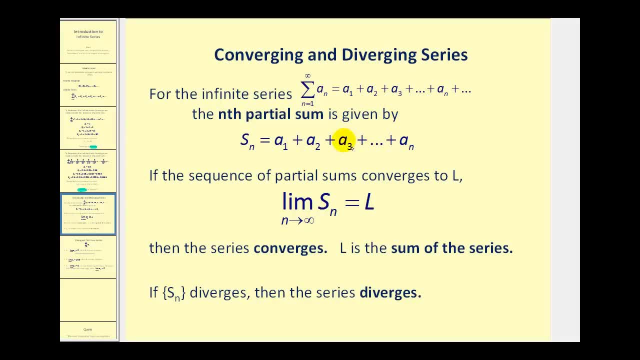 the nth partial sum would be given using this notation, Where s sub n will equal a sub 1 plus a sub 2, all the way to a sub n. If the sequence of the partial sums converge to L, we can say the limit as n approaches infinity of the partial sums is equal to L. 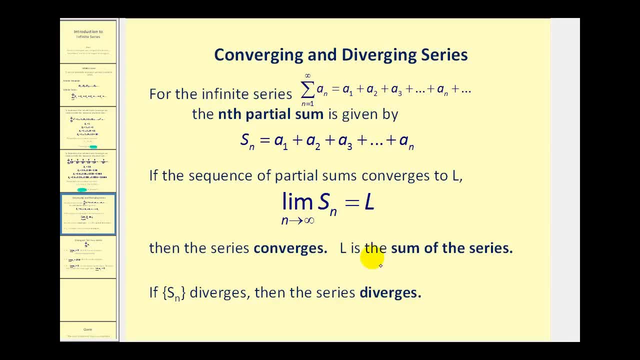 And if this is true, then the series converges. We can also say: the limit L is the sum of the infinite series, And if s sub n diverges, then the series diverges. I do want to mention one more idea for this video. 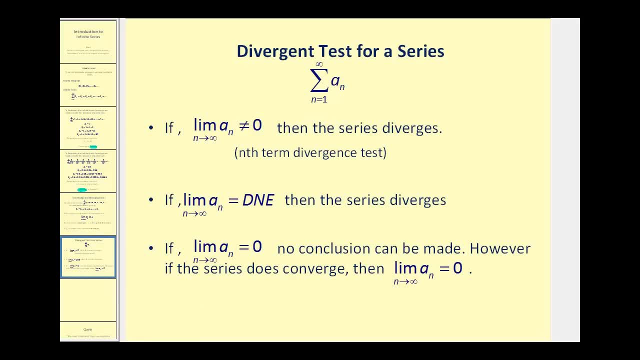 And this is the divergent test for a series. We will see this idea again in many of the other videos. If the limit of a sub n as n approaches infinity, does not equal 0, then the series diverges. Remember, a sub n is the formula that generates the terms in the series. 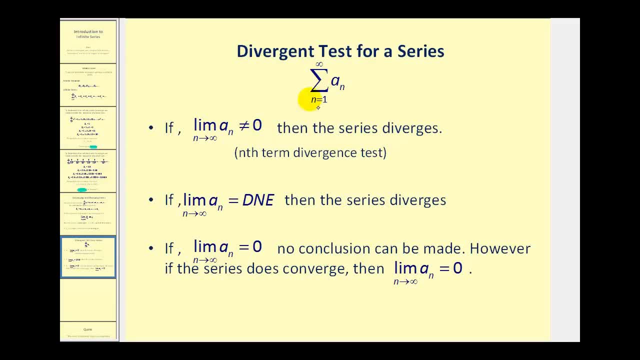 So this is telling us that if the terms don't approach 0 as n increases to infinity, then it's guaranteed that series will diverge. Hopefully that makes sense, because there's no way an infinite series can converge if we're adding numbers that don't approach 0. 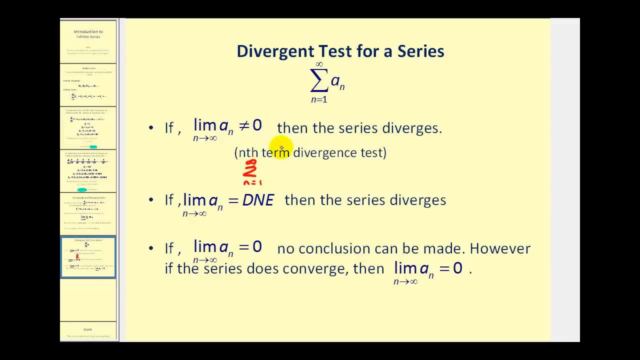 So, for example, if we have the infinite sum of, let's say, 3n divided by n and we take the limit of a sub n, this limit would equal 3.. And since this limit doesn't equal 0, we could say that this infinite series diverges. 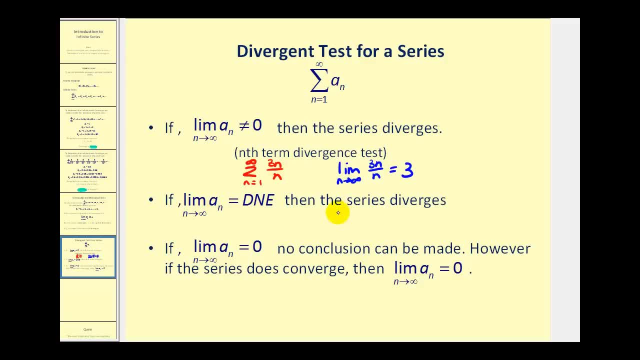 Now it's also true that if the limit of a sub n doesn't exist, then the series diverges. So, for example, if we had the infinite sum of just 3n, well we know the limit, as n approaches infinity, of 3n is equal to infinity. 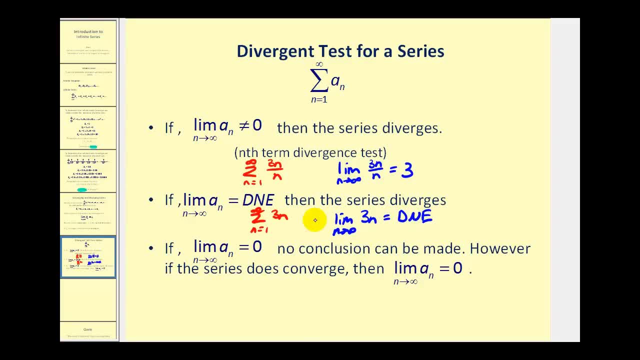 which doesn't exist, and therefore this infinite series diverges. And then, lastly, if the limit of a sub n equals 0,, no conclusion can be made. However, if the series does converge, then the limit of a sub n, as n approaches infinity, must equal 0.